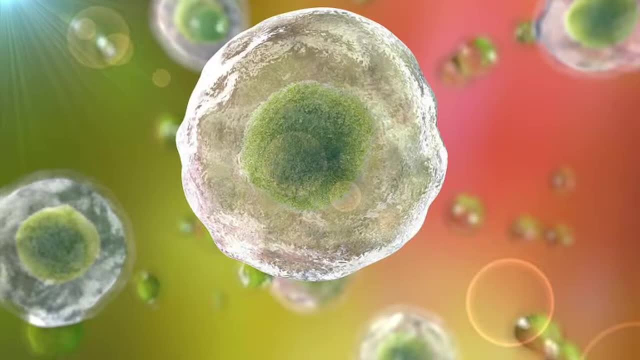 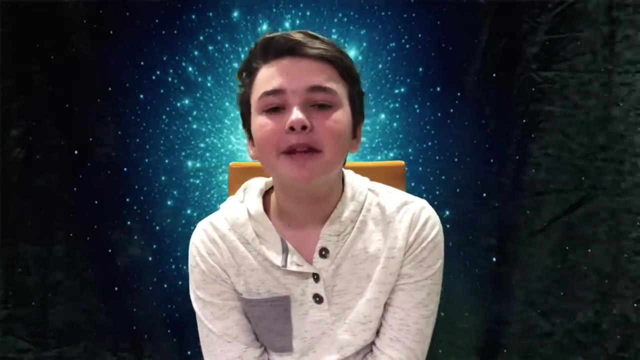 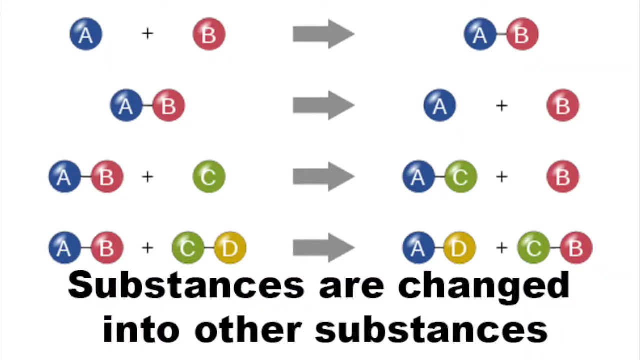 In each cell, thousands of chemical reactions are being taken place. I have a video of chemical reactions. Click up the i in the corner to check it out. Anyways, chemical reactions are processes where substances are changed into other substances- Everything from cooking an egg to baking a cake. 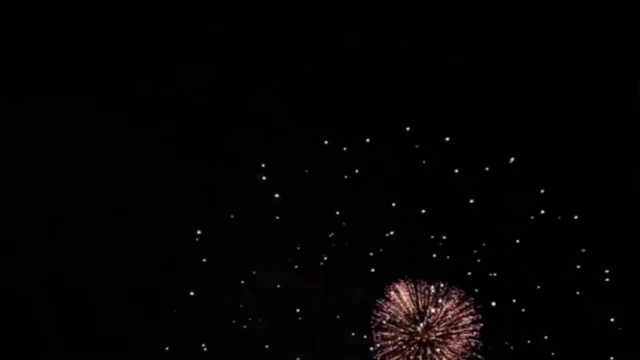 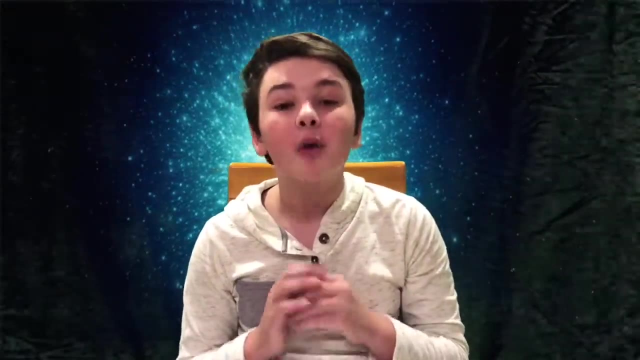 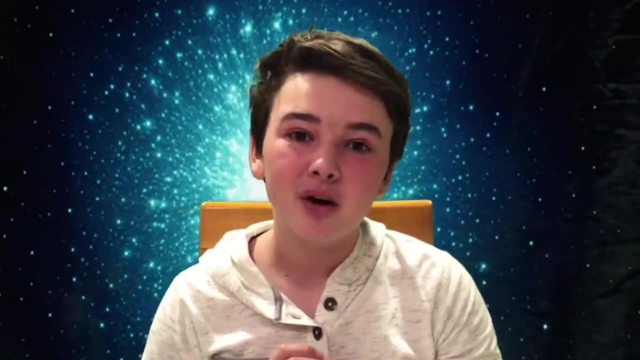 to cooking a cake. Fireworks are all chemical reactions. Like I said earlier, THOUSANDS of chemical reactions are being taken place in every single cell in our body, But some chemical reactions are so slow that they can't get the job done. 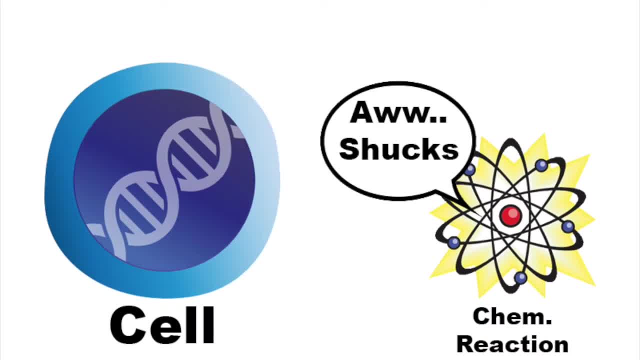 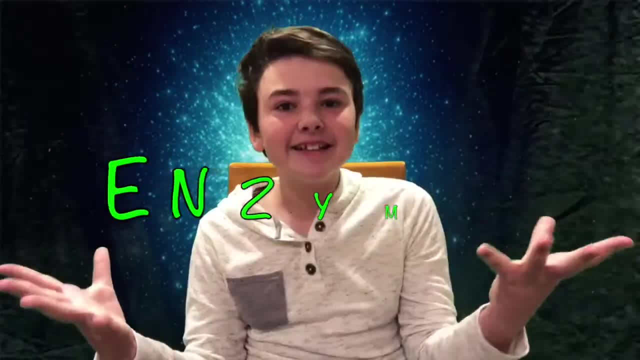 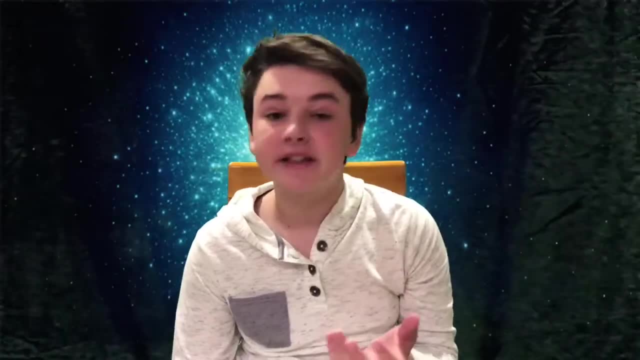 You're fired. Ah shucks, boss. To help these chemical reactions speed up their jobs in our cells, we've got ENZYMES. It's Super Enzyme. Enzymes are proteins that accelerate chemical reactions in our bodies. 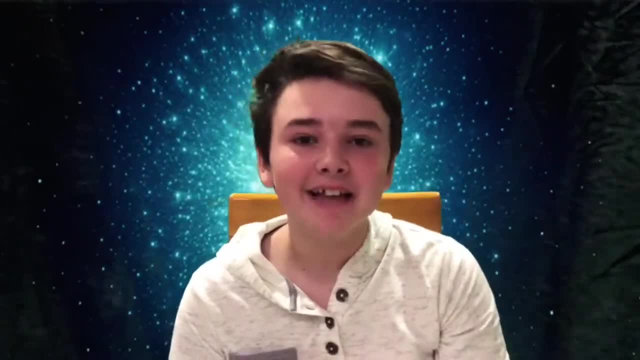 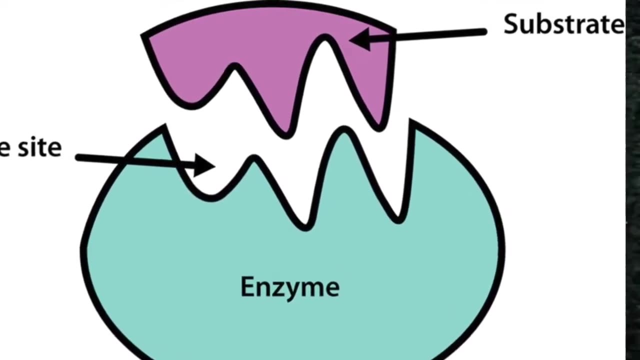 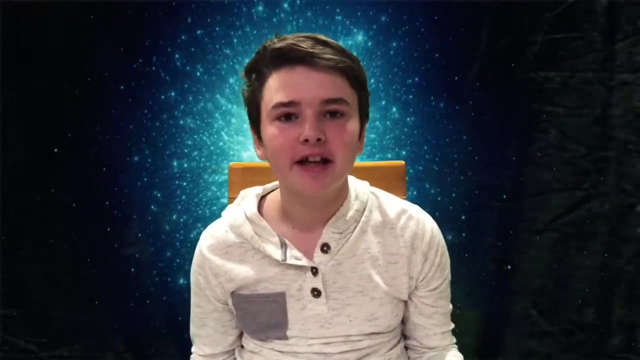 Almost all chemical reactions in our cells need enzymes. Enzymes attach to substances called the substrate. For an enzyme to attach into a substrate, a certain amount of energy is needed. This energy is called the ACTIVATION ENERGY. Our cells get this energy when we eat. 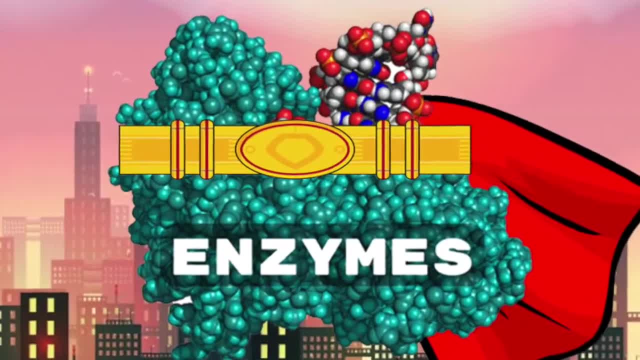 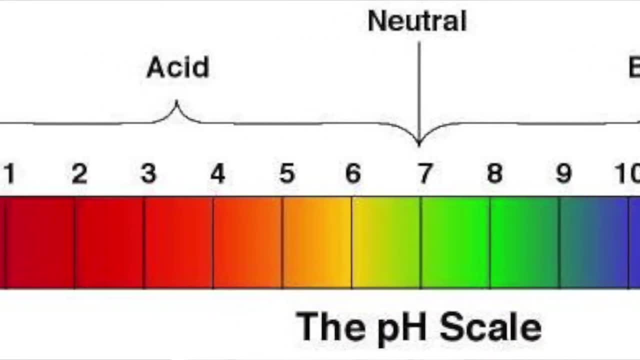 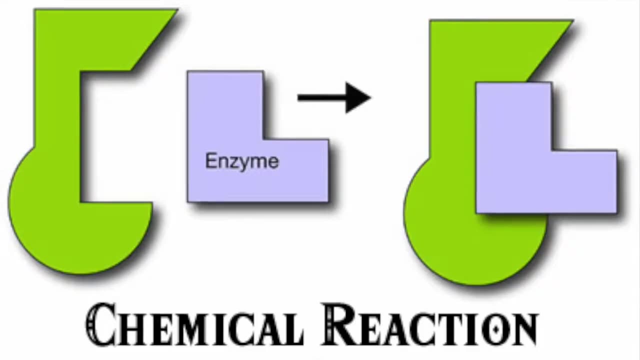 Yum. Also, enzymes work best in certain temperature, certain pH levels, which means just how acidic the area is around the enzyme, and the enzyme shouldn't be overcrowded with too many substrates. With the enzyme's help, the substrates undergo a process called the ACTIVATION ENERGY. 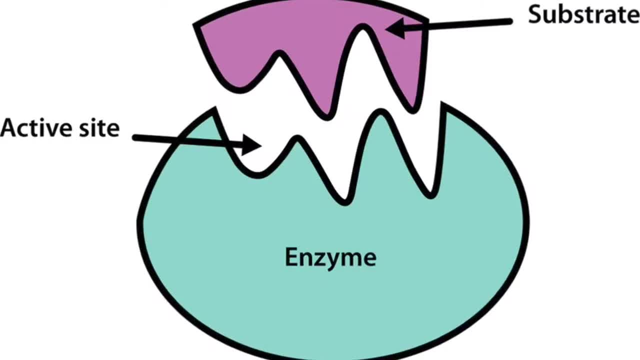 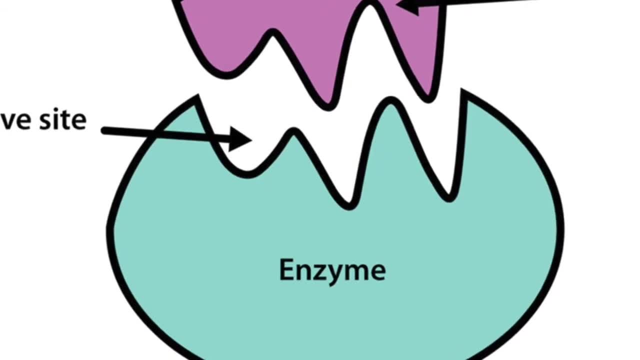 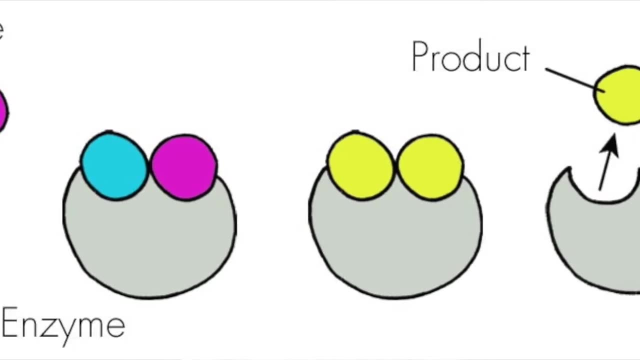 These substrates undergo a chemical reaction. However, every enzyme is specifically made to collide with only certain types of substrates. After the reaction is finished, the substrates turn into products and fly away, and the enzyme stays and gets ready for its next job. 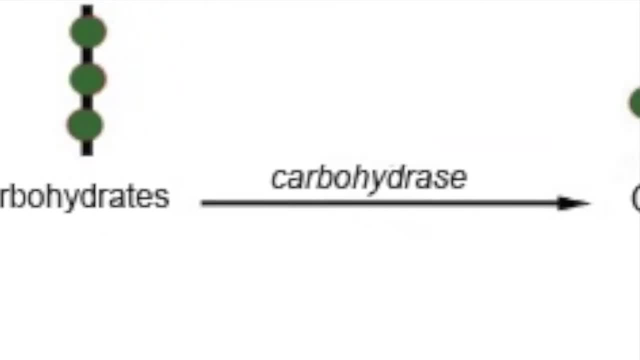 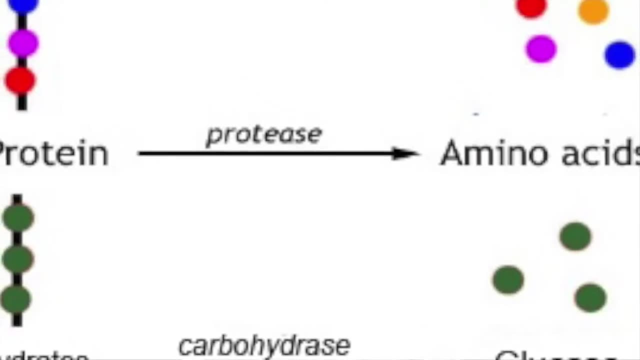 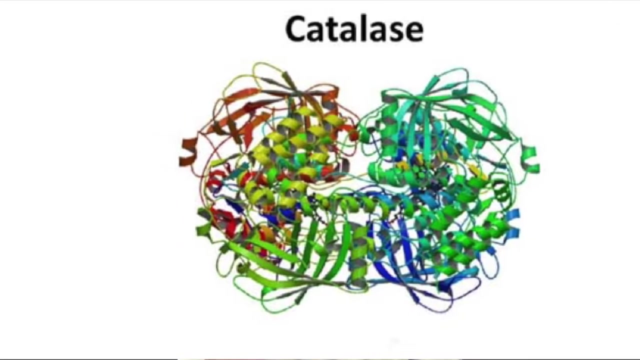 For example, the enzyme CARBOHYDRASE breaks down carbohydrates into glucose And the enzyme PROTEES breaks down proteins into amino acids. Another amazing enzyme is CATALASE. Catalase enzymes break down a substance called hydrogen peroxide into water and oxygen.